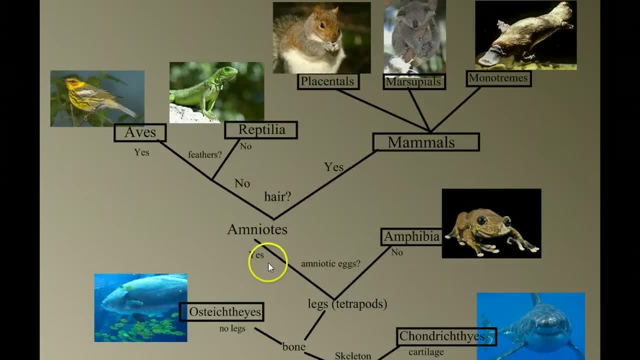 Welcome to our fourth video in our series on vertebrate diversity. In our last video we looked at the amphibians. Now we're going to head down the branch of the amniotes, those vertebrates with the amniotic egg. All reptiles, birds and mammals are considered amniotes. We're going to talk a lot about what amniote means in this video, But let's finish kind of working through our classification key. If a vertebrate has, let's go back down here- has a job. 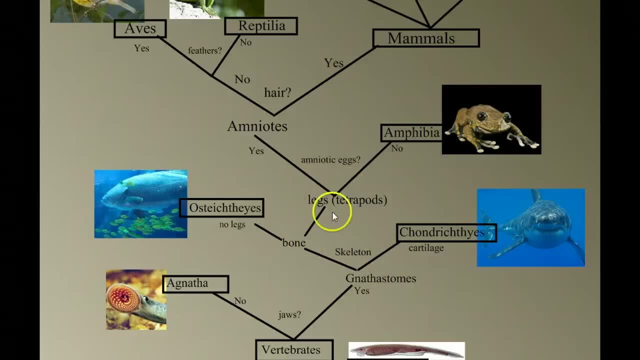 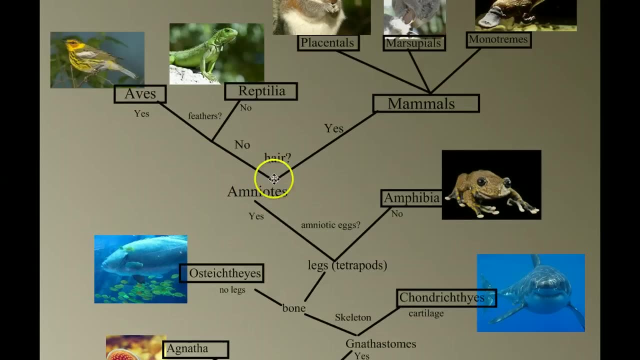 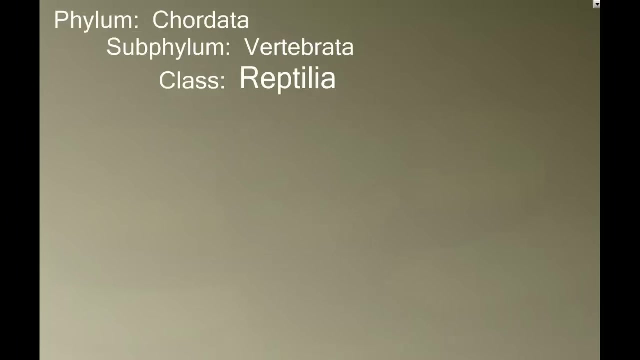 has a jaw, has a skeletomative bone, has legs and has an amniotic egg. it's an amniote. The next question we need to ask ourselves is: does this animal have hair? If the answer is yes, we go to mammals. If the answer is no, we go this direction. And if we go this direction, we have to ask an additional question, and that is: do we have feathers? And if the answer is no, then we are at the reptiles. So in this video we're going to talk about the phylum chordata, subphylum vertebrata class reptilia. 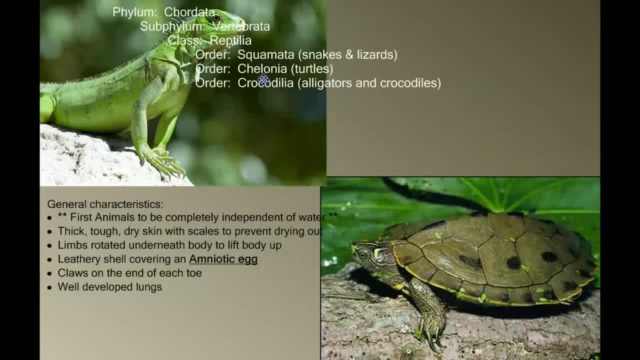 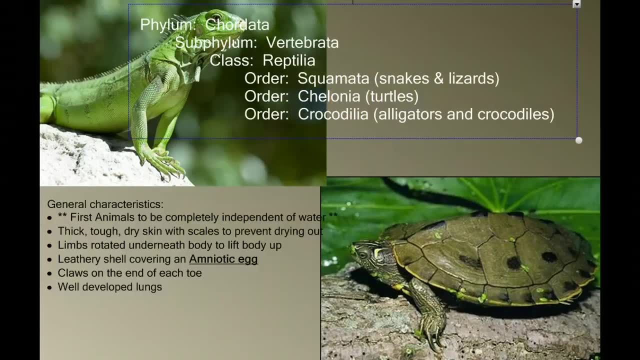 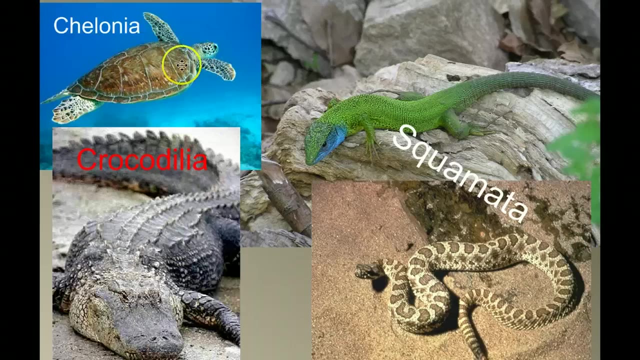 In the class reptilia there are four orders. We're going to study three of them: Order Squamata, Chelonia and Crocodylia. The Squamata include the snakes and the lizards, The Chelonia are the turtles and tortoises, And the Crocodylians include the crocodiles and the alligators. 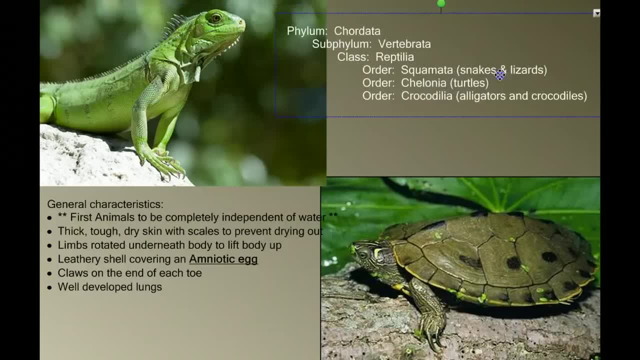 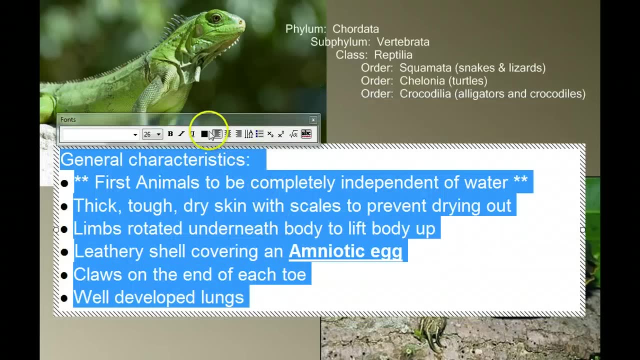 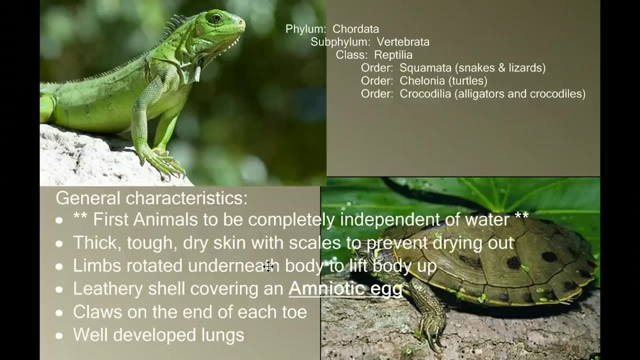 Now, when we look at reptiles, the first thing we need to look at is kind of the general characteristics And the. the reptiles are the first animals that we're going to look at that are completely independent of water. Now, as soon as I say that, you're going to think of many types of reptiles that spend their lives in and around water, But that's not what we mean by independent of. They don't require water for their life cycle. They are terrestrial animals. They lay their eggs on land. When we look at the characteristics of the reptiles, we see many of them that relate to this adaptation. 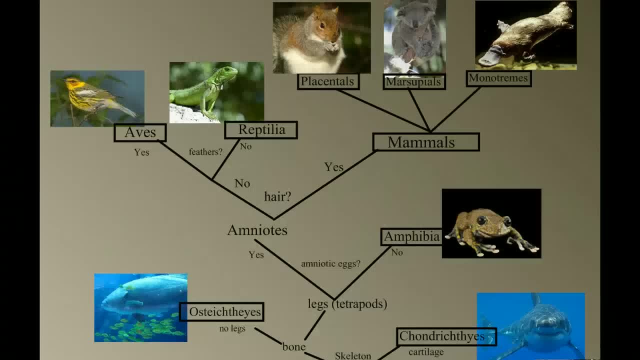 And if you think back to our video on amphibians, we talked about amphibians being our transitional animal, our animal that talk to as we move from the water. you know, everything down here is in water And the amphibians are kind of in between, because they have to start their life in water and then move on to land. But everything from here and up are terrestrial animals, even those that live in and around water. Of course we'll have some aquatic mammals, but we'll address that when we get there. So let's look at some of these characteristics that relate to this adaptation. 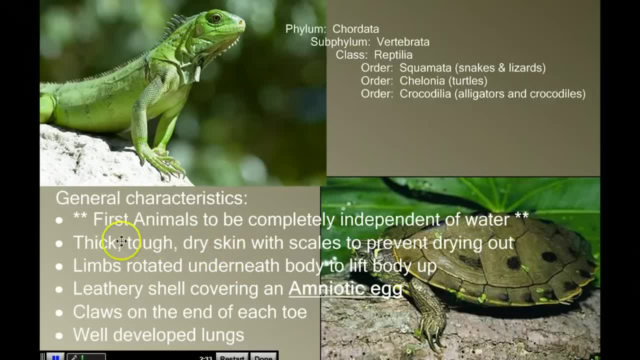 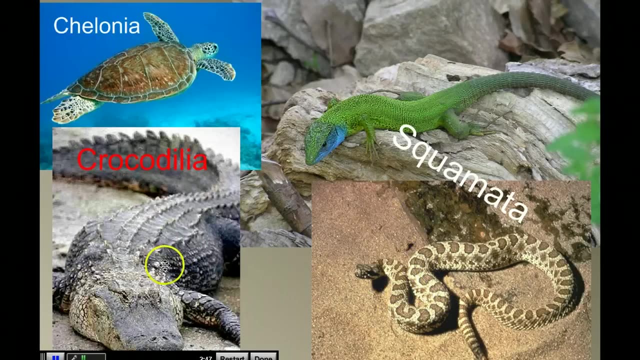 So let's look at some of these characteristics that relate to reptiles being successful on land. They have a thick, tough, dry skin with scales to prevent drying out. We're going to prevent desiccation. You can see this lizard skin here that scales And if we go back to this picture, we can see these scales, these thick scales overlapping, that prevent water loss, And that's a direct adaptation to being successful on land. We've got to prevent loss of water to the dry environment. 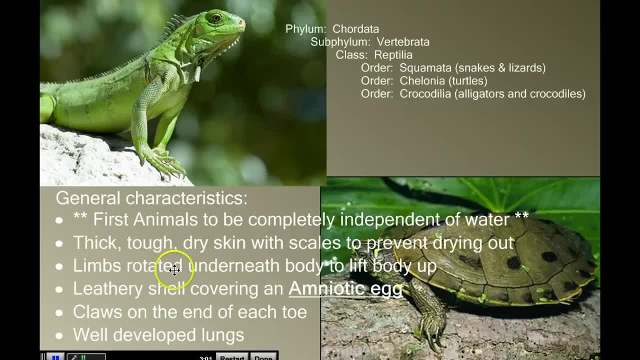 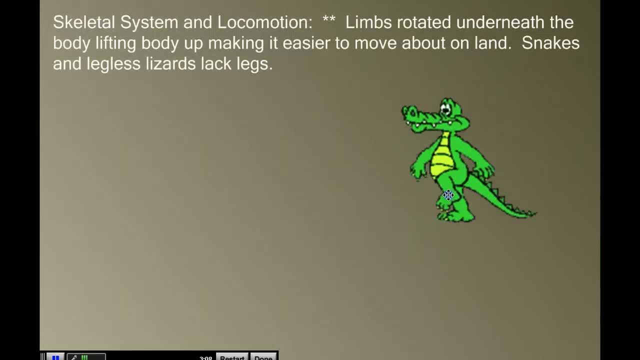 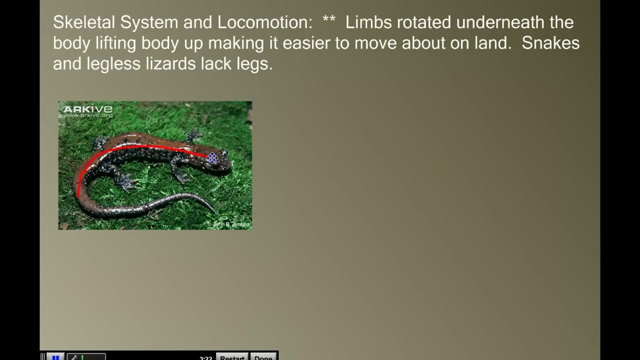 So let's look at some of these characteristics that relate to reptiles being successful on land. So let's look at some of these characteristics that relate to reptiles being successful on land. We've got to prevent loss of water to the dry environment And that's a direct adaptation to being successful on land. We've got to prevent loss of water to the dry environment. 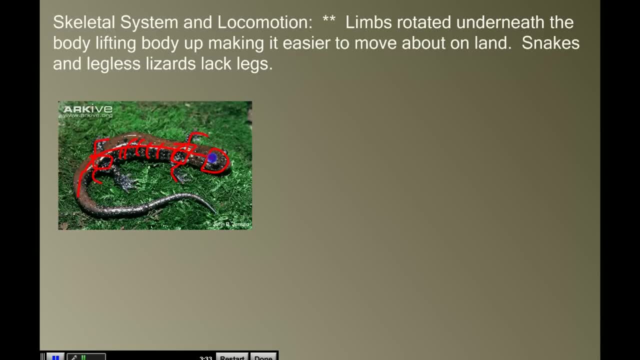